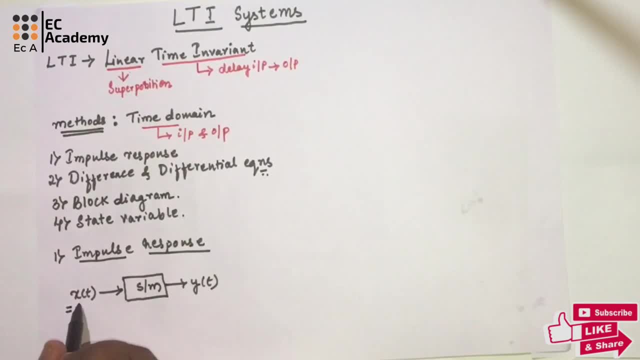 if the input of the system is delta of t, so x of t is equal to delta of t, then the output of the will be equal to the impulse response h of t. So the input is known as impulse and output of the LTI system is known as impulse response. 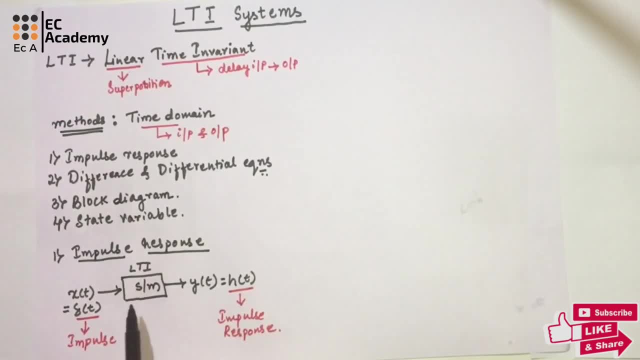 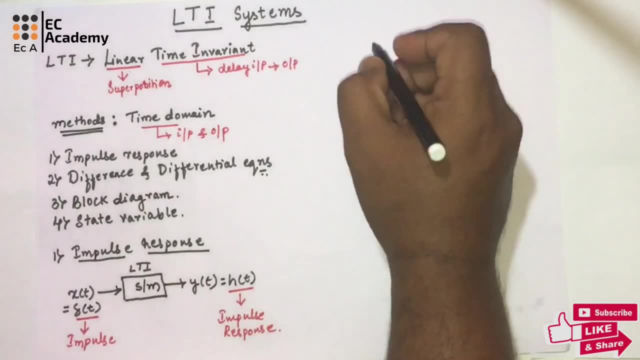 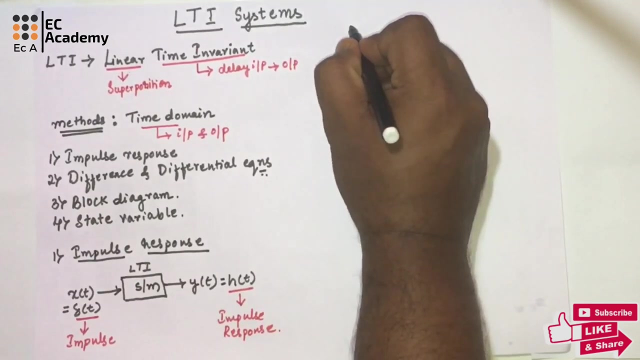 So the characteristics of this LTI system can be studied in terms of impulse response that is defined at the output of an LTI system. Now, if we consider an LTI system, if we consider an LTI system and if the impulse response of the system is given impulse response, 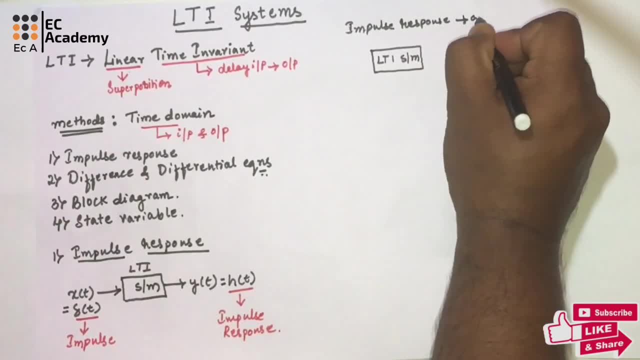 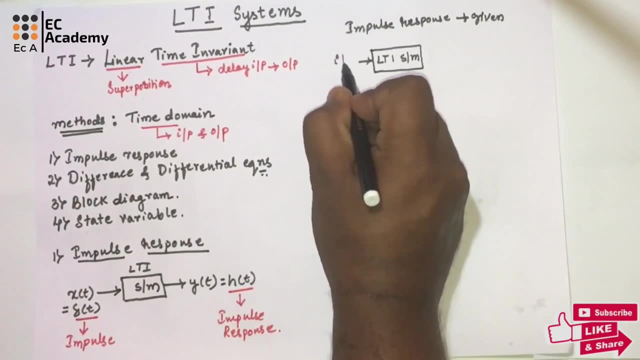 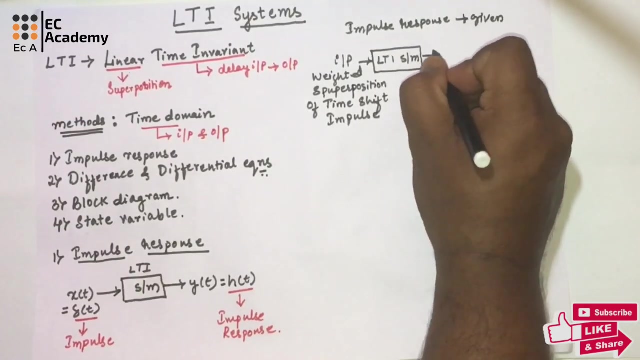 of the system is given. if they have given the impulse response of the system, then if the input is, if the input is weighted- superposition of time shift impulse, if the input is weighted superposition of time shift impulse, then we can find the output of the lta system and this output should also be. 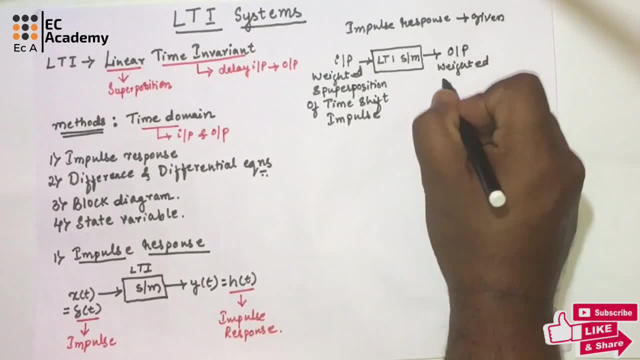 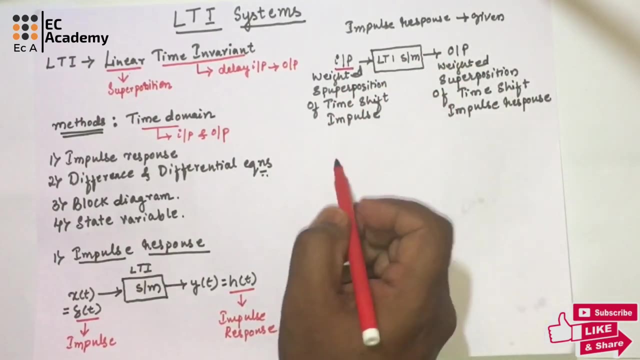 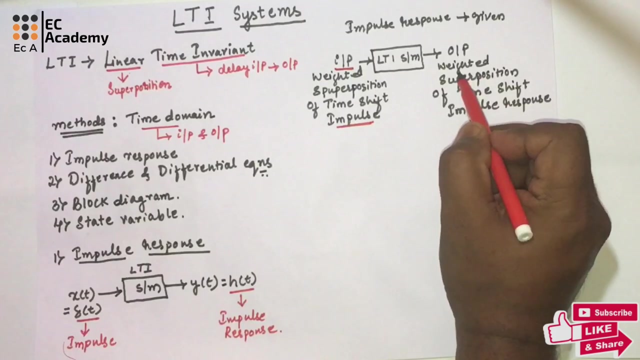 the weighted superposition of time shift impulse response. so here we are taking an input which is weighted superposition of time shift impulse. so we know impulse is the input to the lti system. then the output of this lta system should be the weighted superposition of time shift impulse. 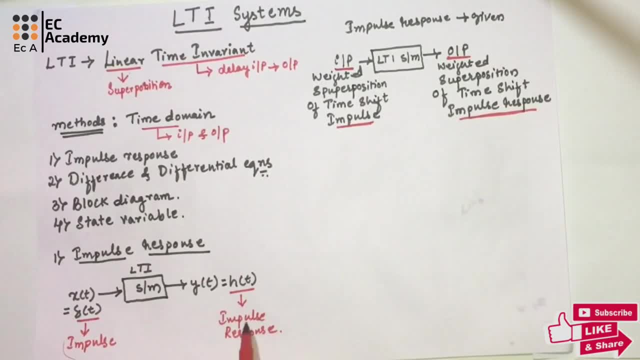 response. we know the impulse response is the output of the lti system. since it is an lti system, if the input is obeying the principle of superposition and time shift, then the output should also obey the principle of superposition and time shift. that's why we call this as an lti.